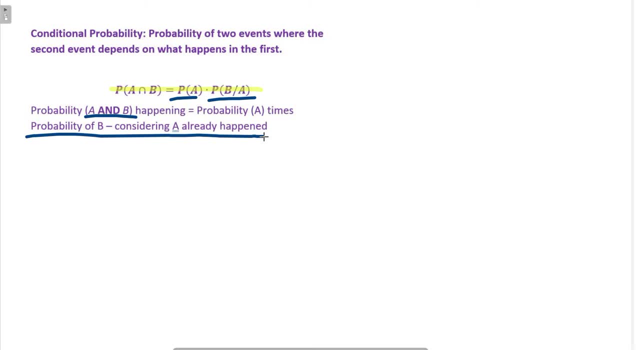 say: okay, I need the probability of B, So B has to be calculated, knowing that A already happened, Something specific already happened. And here's another thing I want to point out: Anytime you have the probability of something and something else, so A and B, as opposed to A or B, you are going to multiply, So let's. 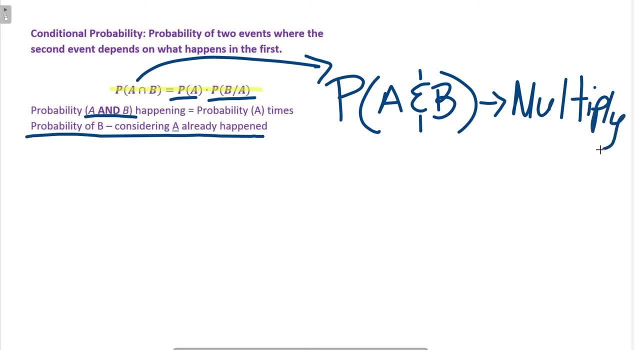 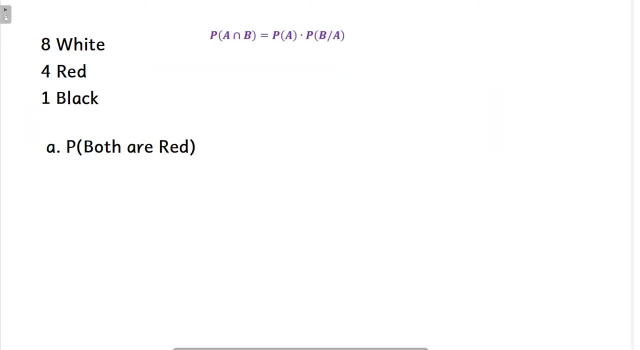 keep that in our minds, All right. So let's get into this. We have the first thing and I've kind of simplified it. on the next screen We have eight white, four red, one black. I've got the formula up here. 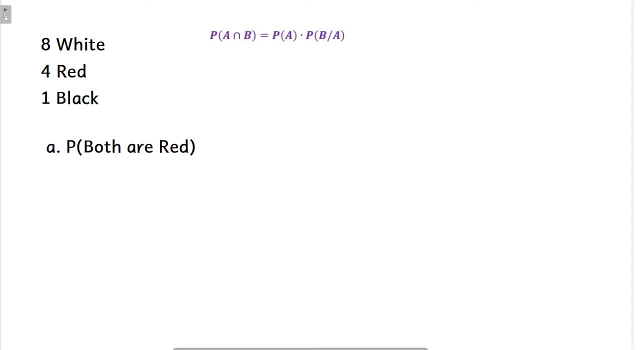 But we're really not going to use it. It's just for your reference. Okay, So the probability that both are red. So what I want to do is I first want to make the probability of both things So probability of A happening. Okay, Let's see, We have eight plus four, That's. 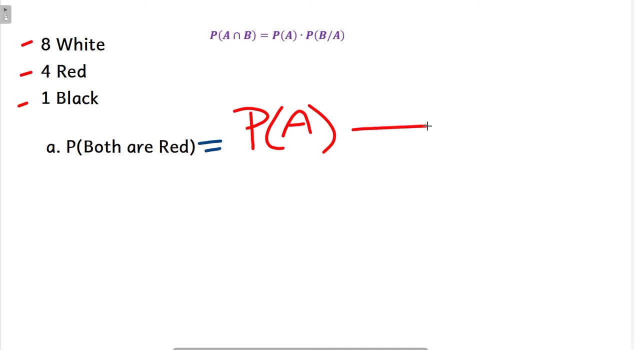 12 plus one, We have 13 total. So remember, probability is the numerator is the number of times the thing you want to happen can happen, And the denominator is the total outcomes. So there's 13 total marbles in this jar. 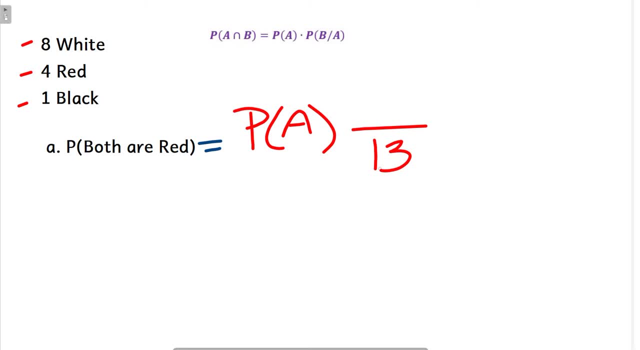 Okay, And only eight of them are red. Nope, Only four of them are red. Okay, So four out of 13 is the probability of A happening. All right, So the next thing is probability of B. So let's look at the probability of B. Probability B is also red because both are. 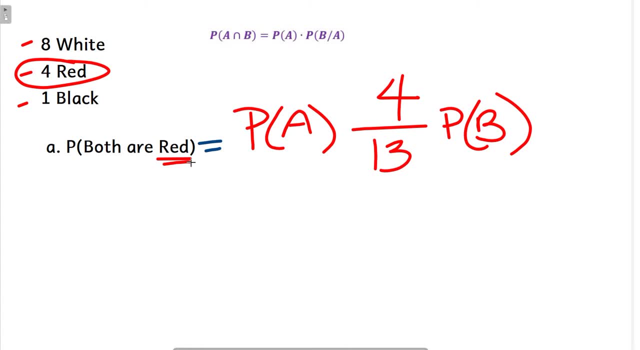 red. So our probability is not the same. Remember that A already happened. So what has happened? I picked a red marble out of this jar. I've set it aside, So there are no longer four red marbles in the jar And there are no longer 13 marbles. 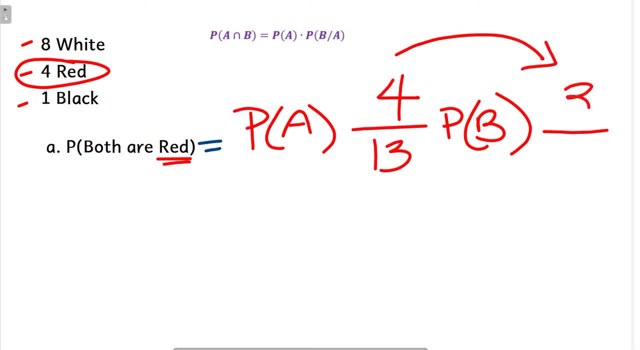 There are now 13 marbles in the jar. There are now three red marbles- because I've chosen one out and I didn't put it back- And then there are 12 total. Okay, So we have four thirteenths and three twelfths. So let's go and multiply these. Let's actually do something. 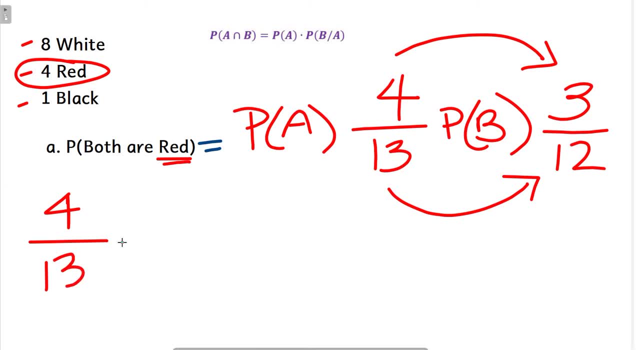 to help ourselves out a little bit. We have four thirteenths times instead of three twelfths. if we divide both of those by three, we get one fourth Right, And then we can go ahead and divide out here. You can go ahead and multiply it. 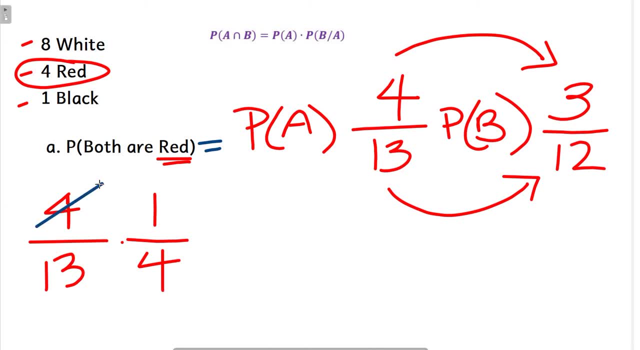 You can multiply if you want, But I really wouldn't Divide. four goes into four. one time. When you multiply fractions, remember we multiply straight across And we get one over thirteenth as our probability. Okay, So we're going to do this two more times And the process really 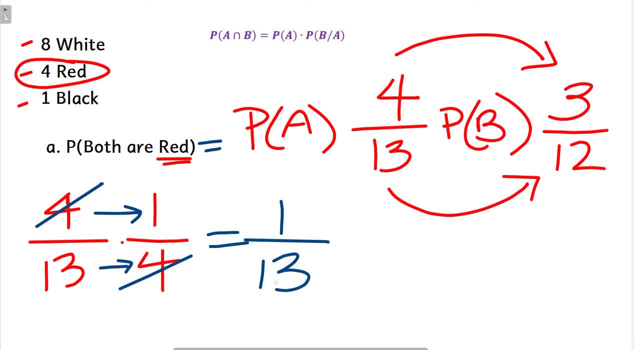 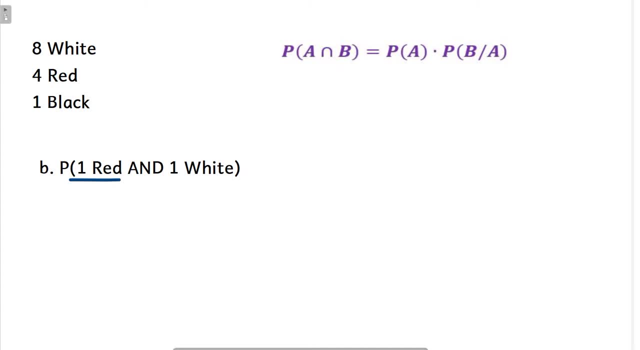 isn't going to change much. We're just going to change those probabilities that we find. So let's go to the next screen. All right, This time we want the probability that there's one red. We keep that out, And then, when we go and choose another, we get a white All. 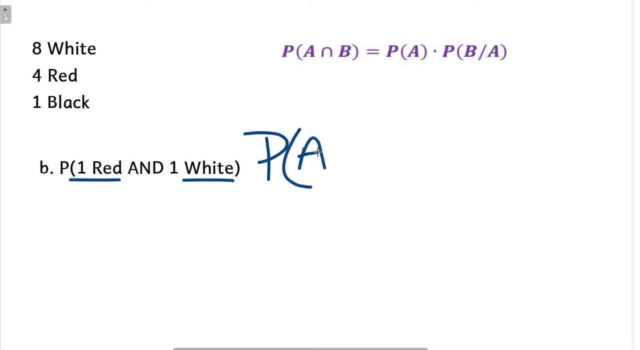 right, So let's do the same thing we did before. Probability of A happening is: well, there's four reds, Remember. this is a different situation. Thirteen total Probability of B happening: All right, Well, we're choosing a white. We haven't chosen a white yet, So 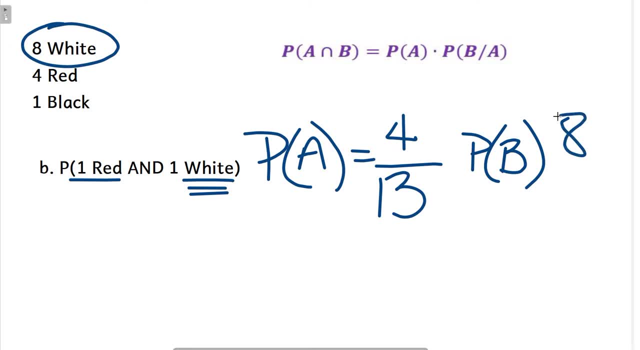 there are still eight in the jar. So there's eight, That doesn't change, But there are no longer thirteen in the jar, There are now only twelve. Okay, So four thirteenths times eight twelfths is how we're going to do this. 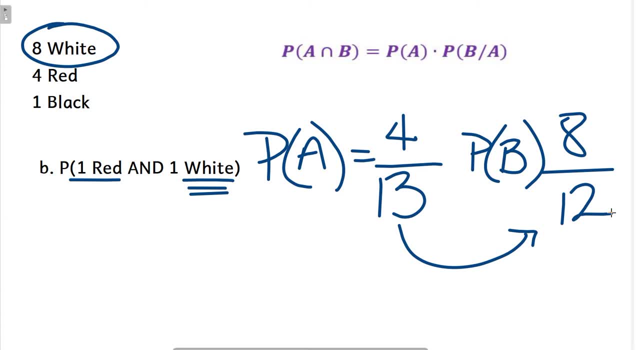 And remember: I really think you should simplify these fractions. Don't make ugly fractions. Don't multiply ugly fractions if you don't have to. So let's say 4 13ths times and instead of 8 12ths, we're going to go ahead and divide both by 4 and get 2 3rds, okay. 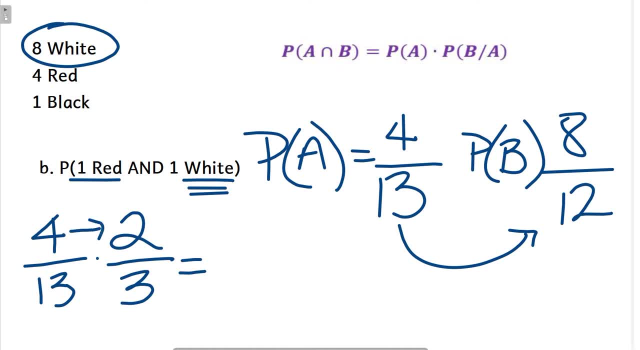 And then we're going to. now we can multiply: 4 times 2 is 8.. 13 times 3 is 39.. Don't believe you can simplify that? That is our answer. Okay, Let's look at the last one they asked us to do, part C. 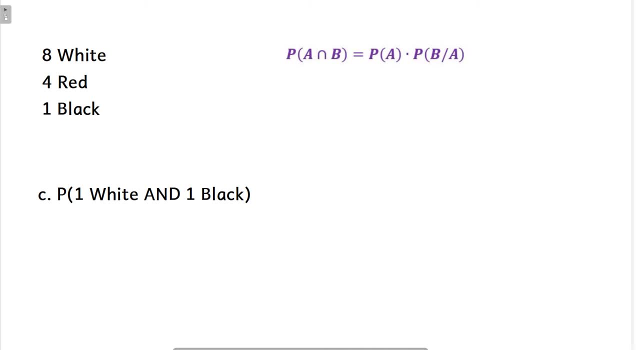 All right, It wants one white. so I pull out two marbles, Remember: one white, then one black, And this because we're not replacing it. it doesn't matter if they asked us to pull them both out at the same time. 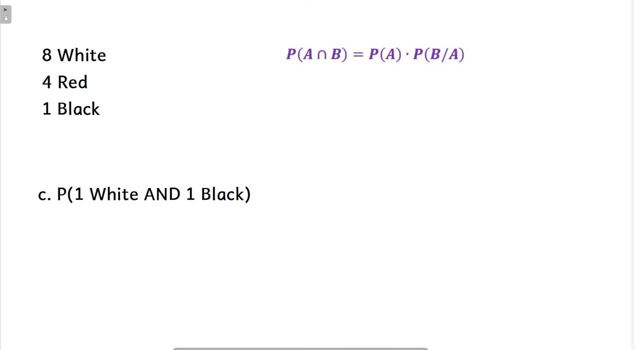 or pull one out and then not replace it and then pull another one. It literally doesn't matter. So we pull out one white. So what's the probability that we get a white marble? Well, let's look. That is 8 possible white marbles out of 3..